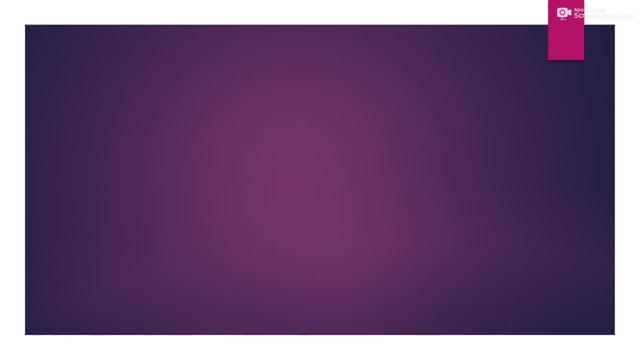 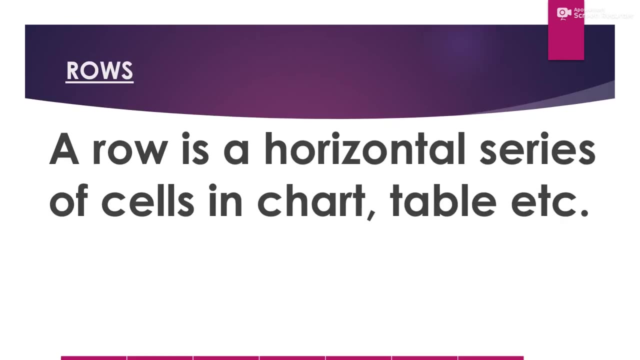 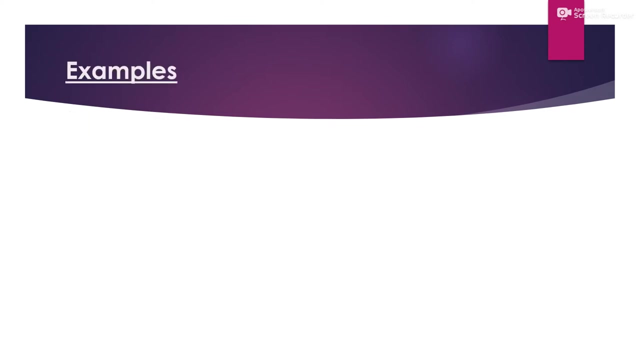 Hello everyone. today's topic is rows and columns. First of all, we will discuss about rows. A row is a horizontal series of cells in chart table, etc. Let us count the rows 1,, 2,, 3,, 4, 5.. So there are total 5 rows. Now we will discuss about columns. 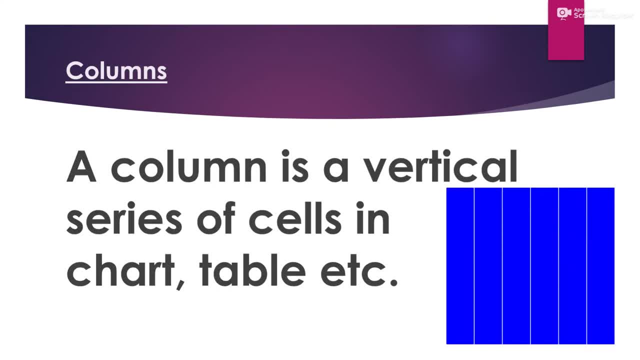 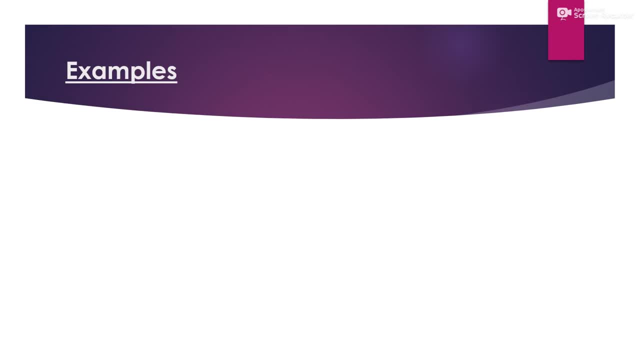 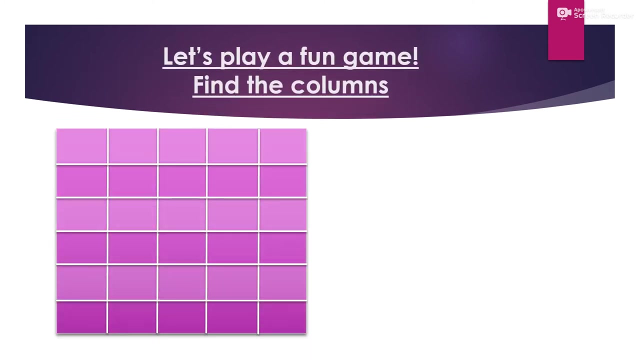 A column is a vertical series of cells in chart table, etc. Let us count the columns 1, 2,, 3,, 4,, 5, 6.. So there are 6 columns. Now let's play a fun game Here. we have to find out the number of columns. 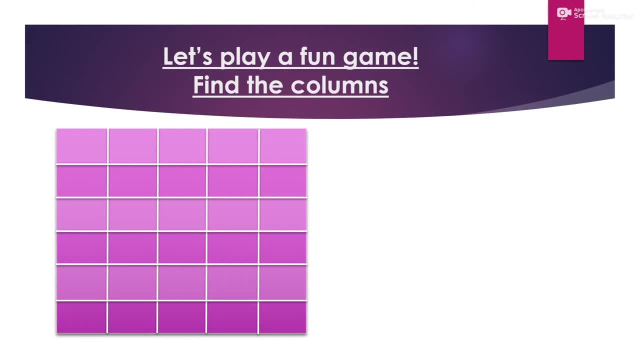 So first of all we will count it: 1,, 2,, 3,, 4,, 5.. So here total 5 columns. A column means vertical series of cells: 1,, 2,, 3,, 4, 5.. 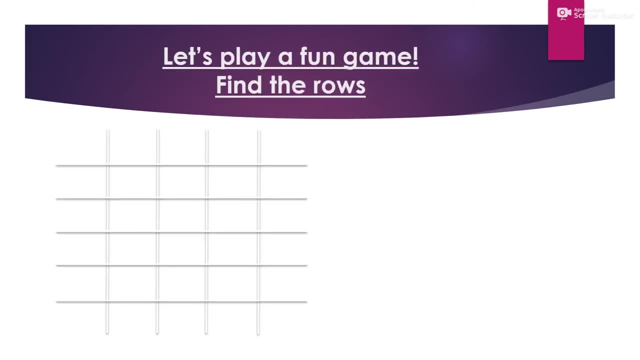 Now we will count these columns. Here we have total 5 columns. Let us add top and bottom rows. Let's add top and bottom rows. We will play a fun game once again. Here we have to find out the rows, So for that we have to count a horizontal series of cell. 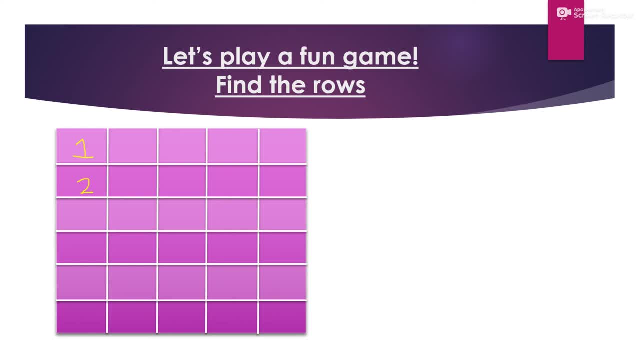 1, 2,, 3,, 4,, 5,, 6.. So there are 6 rows. I hope you have learnt this topic very well, So do practice. Thank you.